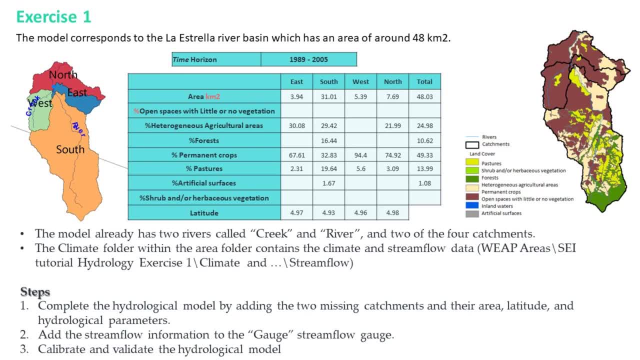 To simplify the exercise in this tutorial, the catchments were disaggregated considering only the land cover classes. The modeler defines the disaggregation which aims to assign hydrological parameters correctly, considering factors related to not only the vegetation, but also geomorphological and geological features. 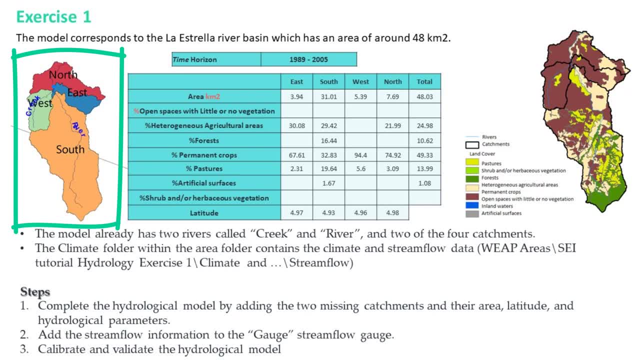 Four catchments were defined. They are shown in the figure in different colors. Areas in square kilometers and percentage distribution by land cover classes in each catchment are shown in the table. The table also shows the central latitude of the polygons representing catchments. 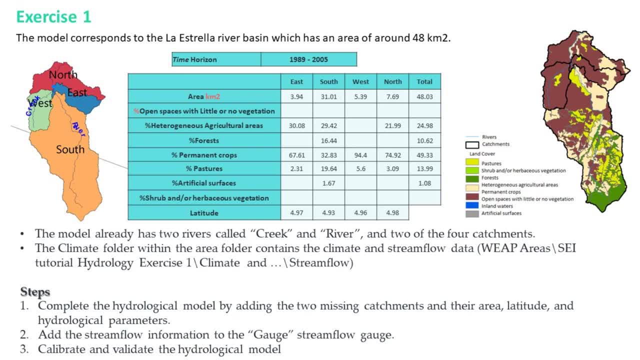 The model already has two river squares- One is called creek and river and two of the four catchments. The climate and streamflow data are in the model folder within the WIP areas folder. We will follow the next steps. First, we need to complete the hydrological model by adding the two missing catchments. 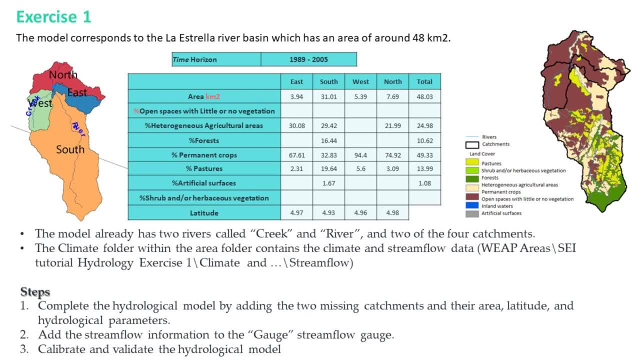 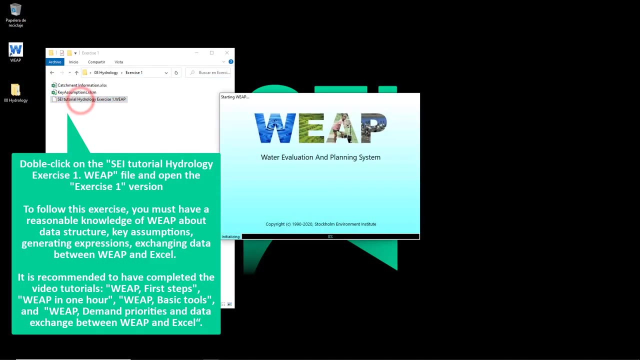 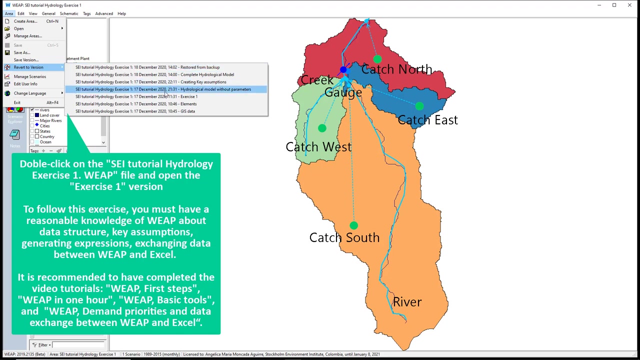 Then we need to enter their area, latitude and hydrological parameters. Next, add the streamflow information to the gauge: streamflow gauge. Finally, calibrate and validate the hydrological model. To follow this exercise, you must open the SEI tutorial hydrology exercise 1 file and open the exercise 1 version. 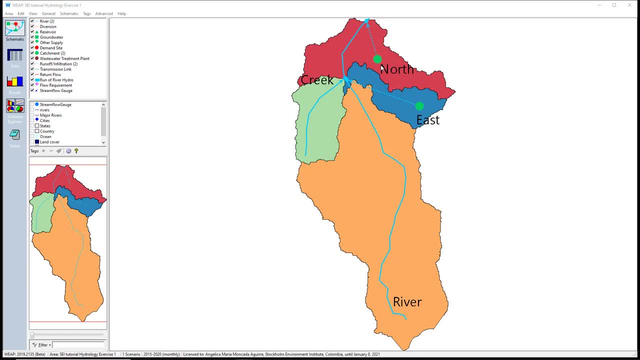 The model has two catchments, two runoff infiltration links and two rivers. We are going to set first the time horizon of the model, Go to general years and time steps. The modeling period is from 1989 to 2015.. It is a monthly model, meaning one year is divided into 12.. 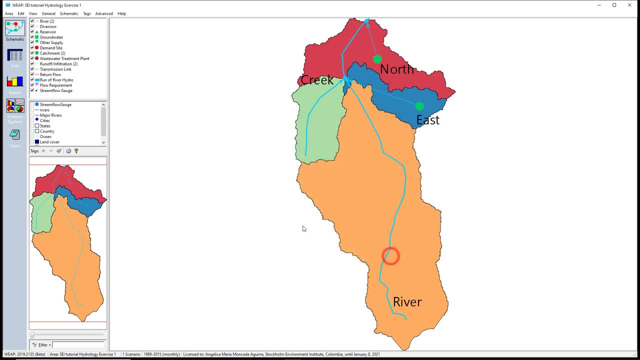 To complete the schematic of the model, we need to add two catchments and the streamflow gauge. The modeler assigns the names of the catchments. I prefer to add the prefix catch to distinguish them from the demand sites in the data tree. 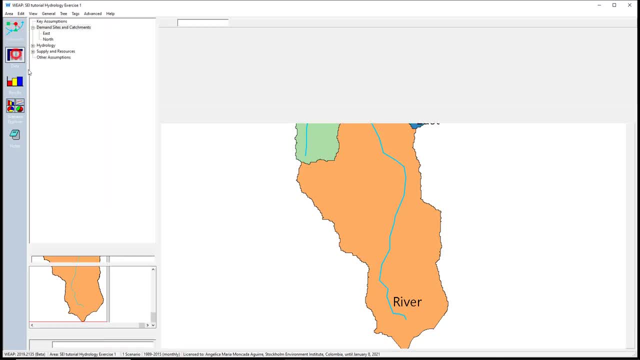 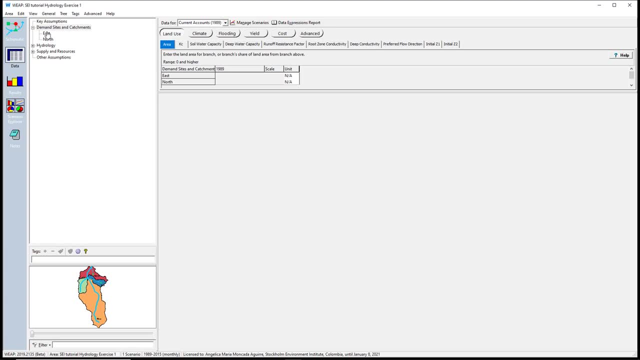 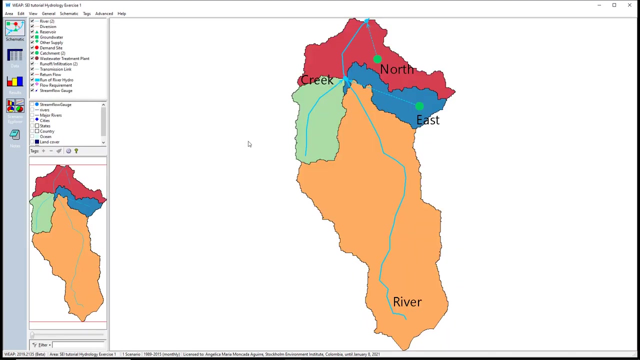 WIP groups catchments and demand sites under the same category. in the data tree Assigning the prefix catch, we can sort by name and differentiate them. These elements are grouped because a catchment can also include an irrigation demand. We will name the catchments with the prefix catch, followed by their location. 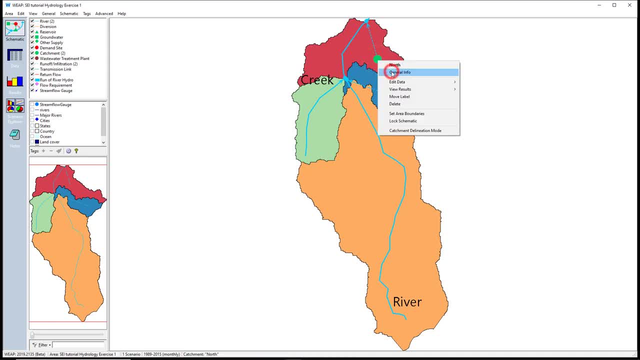 Right click on the north catchment, select general info and add the prefix catch to the name Finish. Do the same for the east catchment. Right click general info, catch, east, finish. We are going to add now the two missing catchments. 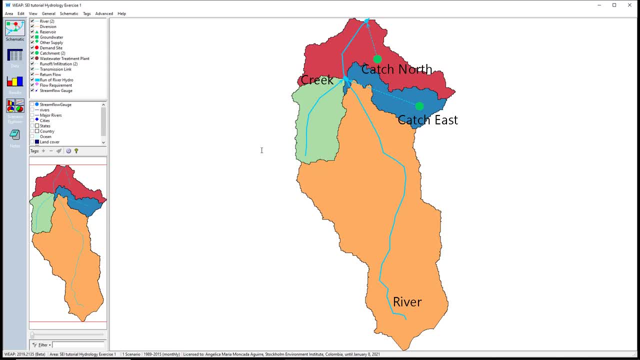 WIP elements are added by dragging and dropping to the desired location, if it is represented as a point, or upstream to downstream, if it is represented as a line. Drag a catchment from the element panel and drop it on this orange polygon. There are two ways to add catchments: manually and use the catchment delineation mode. 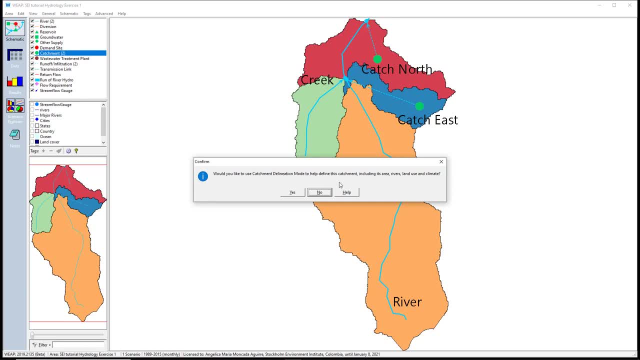 We will use the catchment delineation mode during the third hydrology practical exercise. Click on no for now. Name it: catch south- Finish. Repeat this process for the other missing catchment. Drag a catchment from the element panel and drop it on this green polygon. 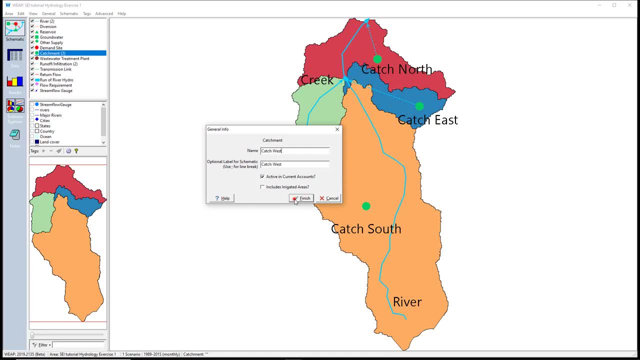 Name it: catch west Finish. If we are going to use the soil moisture method, we must add a runoff infiltration link to each catchment. The end point location defines where WIP will add the catchment's outflows. We will add it to the rivers, but it could also be added to a groundwater node. 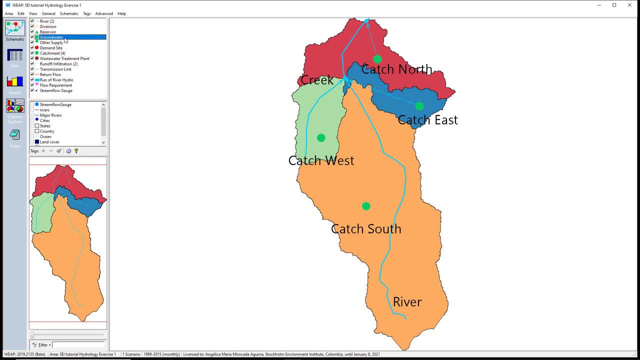 The runoff infiltration link must be plotted following the flow direction from the catchment to the river. Drag a runoff infiltration link and drop it on the catch south catchment. Remember that the end point location defines where the outflows will be added. The end point should be located according to the area representing each catchment. 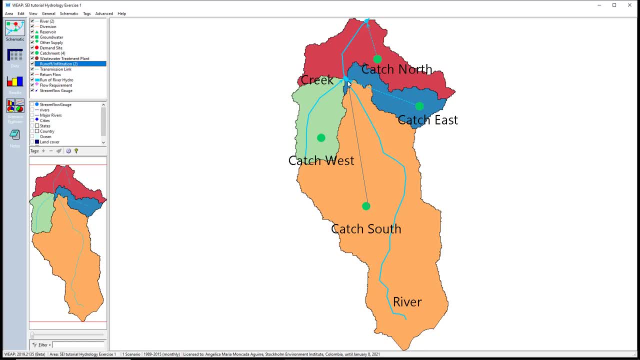 Double click on the river at the poor point of the orange catchment polygon. Here You are asked in the pop-up window: does this catchment inflow represent the headflow for the river's river? If we select yes, the end point will be added to the headflow of this river. 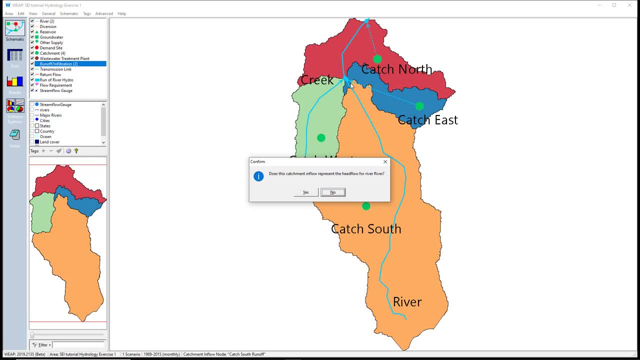 If we select no, the end point will be added where you clicked on Select yes to see what WIP does. If we leave the schematic like this, these catchment outflows will be added here, meaning that they come from a basin upstream of the starting point of this river. 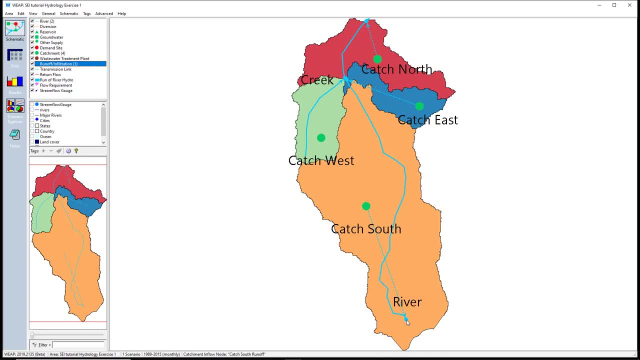 These catchment outflows represent the orange area. Therefore, we must add the ending point here and not at the headflow of this river. We can drag this ending point and move it to where we need it, Drop it here, at the poor point of the orange catchment. 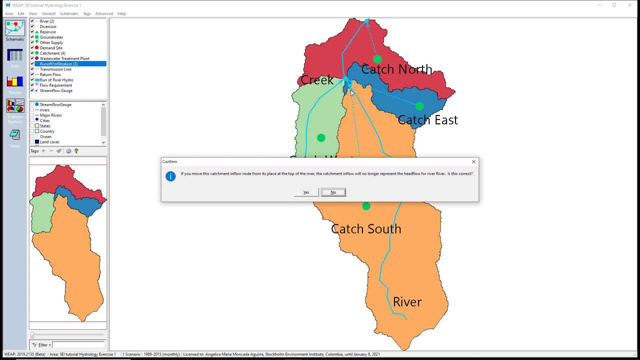 We are asked in the pop-up window: if you move this catchment inflow node from its place at the top of the river, the catchment inflow will no longer represent the headflow for the river's river. Is this correct? 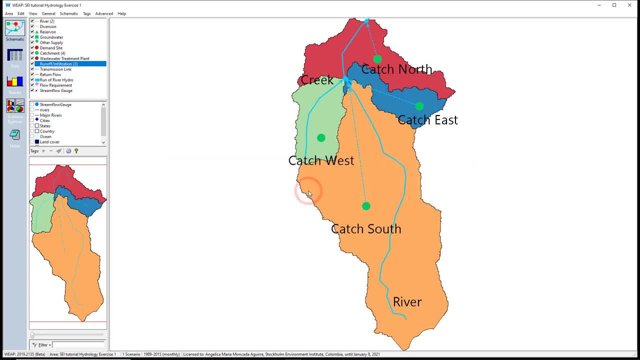 Select. yes, This is what we are looking for. You must add the runoff infiltration links carefully. The model schematic should represent reality as best as possible. This orange area is being represented by this catchment. WIP will calculate the water balance for the entire area. 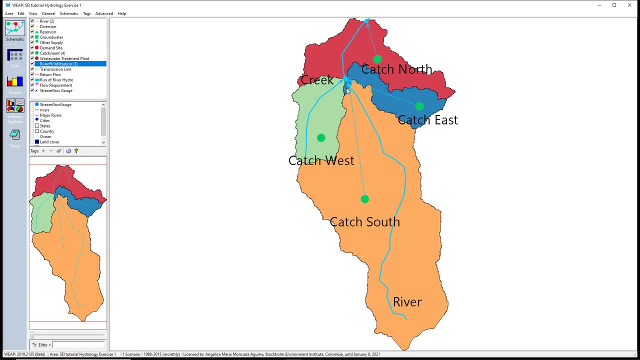 Therefore, flows should be added at the poor point of this area. At this point we will only have natural streamflow results. Repeat the process for the catch west: Drag a runoff infiltration link and drop it on the catch west catchment. Double click on the poor point of this green catchment area. 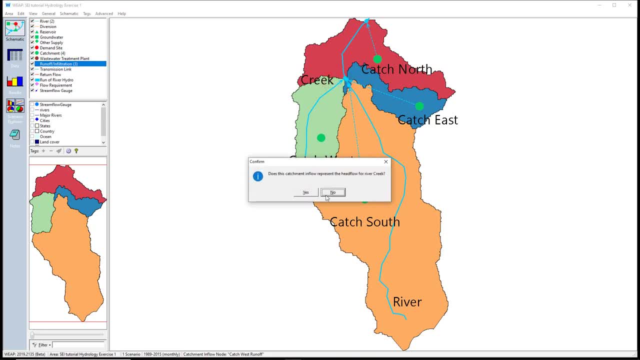 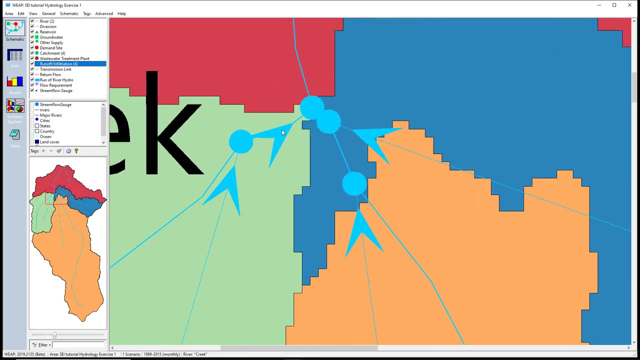 We must select no, because these catchment outflows do not represent the headflow for the river. Zoom in to see how WIP will add the catchment outflows to the river. The outflow from this orange catchment will flow downstream of this inflow node to this river ridge. 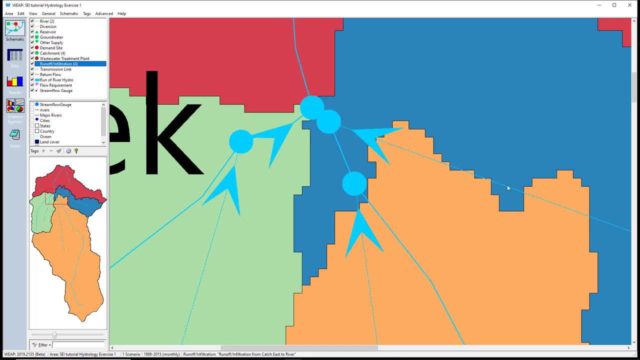 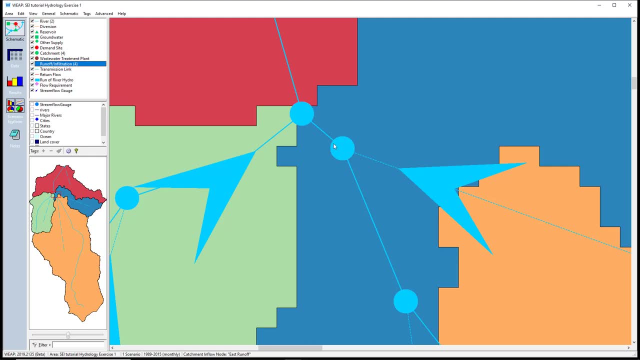 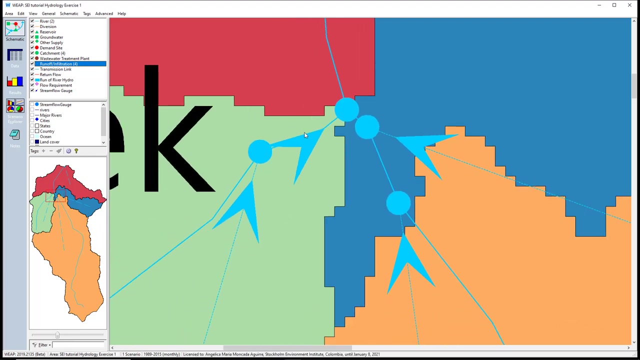 The outflows from this blue catchment will flow downstream from this inflow node. That means that the streamflow in this river ridge will correspond to the accumulated outflows from the orange and blue area. The streamflow at the mouth of this creek corresponds to the outflows of the green catchment. 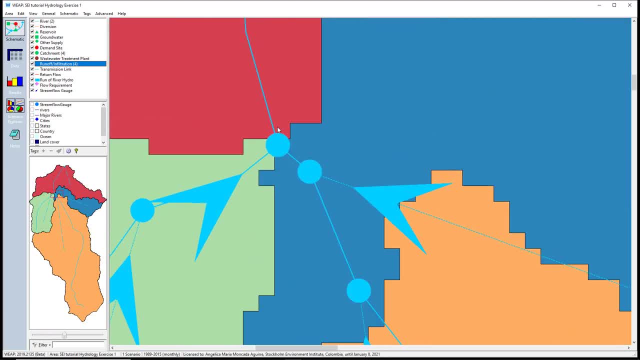 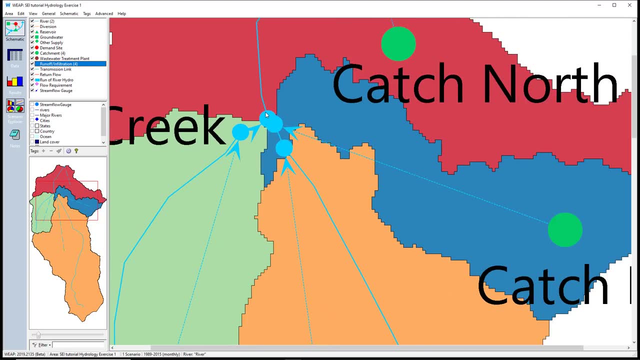 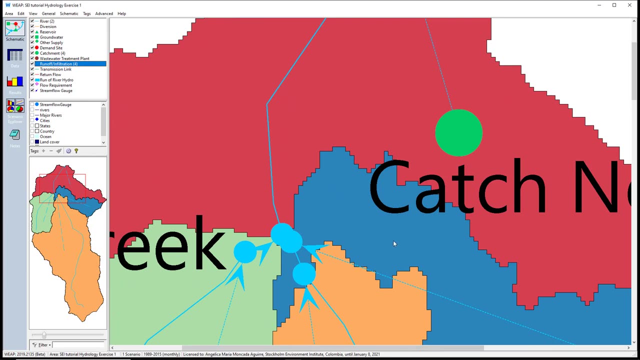 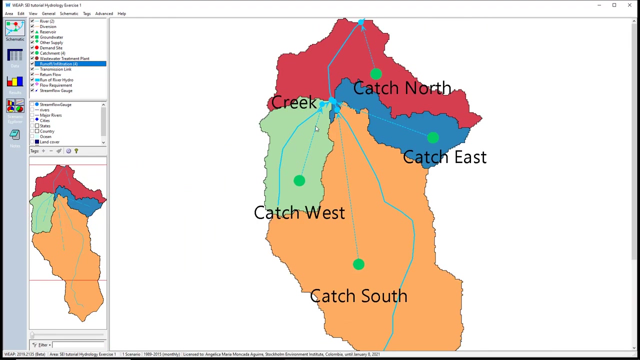 WIP adds the creek streamflow to this river ridge downstream of this inflow point. The streamflow in this river ridge corresponds to the accumulated outflows of the orange blue and green catchments. I am highlighting this because the ending points of the runoff infiltration links, which are inflow nodes, define the river ridges. 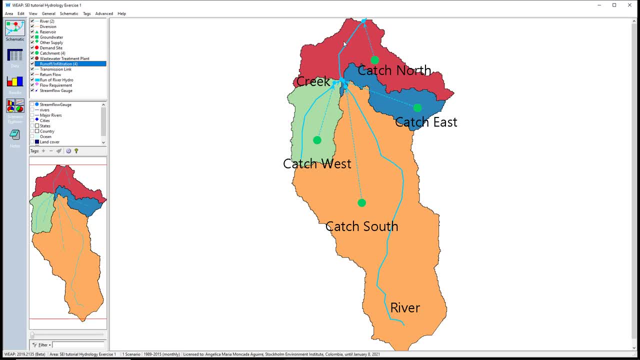 Therefore the streamflow available over each river. The model schematic must reflect the modeling system. The order of the inflow points must be checked. Finally, the only element we are missing on the schematic is the streamflow gauge. Turn on the streamflow gauge layer on the GIS layer panel. 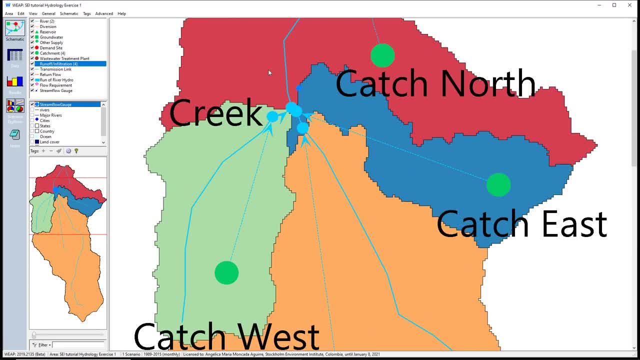 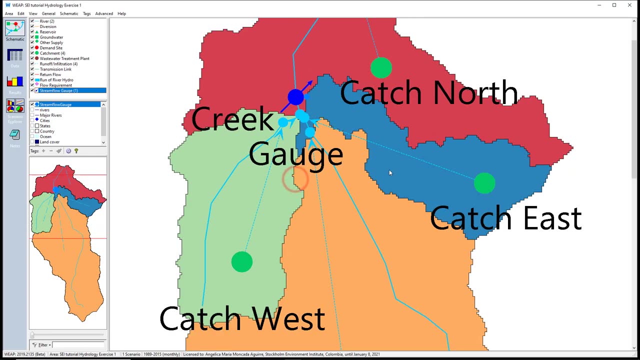 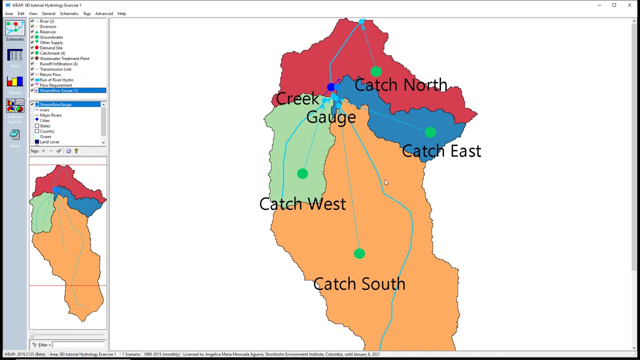 Drag the streamflow gauge element and drop it on the river near this blue point, which represents the location of the station. The streamflow gauge element must be checked. From a schematic point of view, the hydrological model is complete. The model has the rivers, the catchments with their runoff, infiltration links and the streamflow gauge. 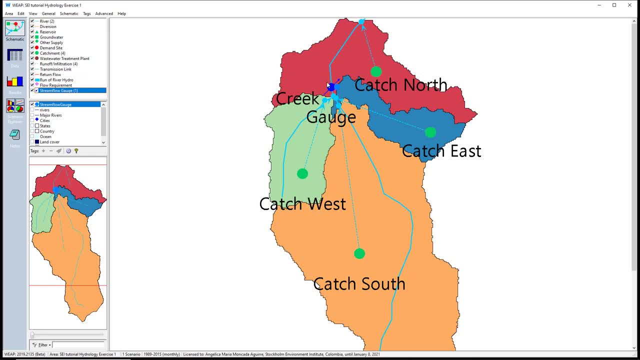 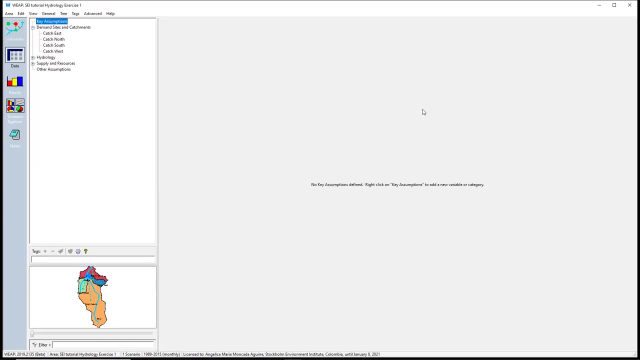 The next step is to characterize each element. We will start entering the streamflow information. Right-click on the streamflow gauge, Select edit data and then streamflow data. We can access any streamflow gauge by going to supply and resources and then river. 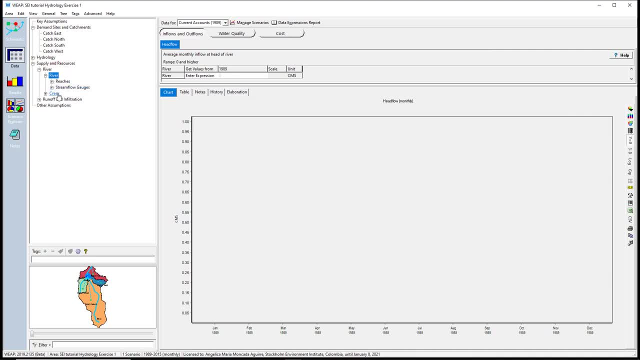 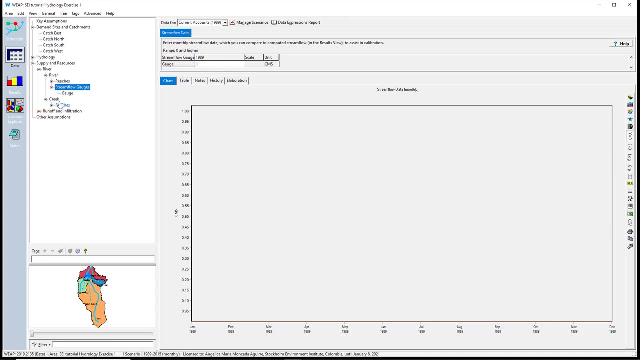 We have two rivers named river and creek. When there is a streamflow gauge on a river, this streamflow gauge category appears. If you expand the tree under the creek, there is no streamflow gauge category. As you build your models, you will become familiar with this structure of the data tree. 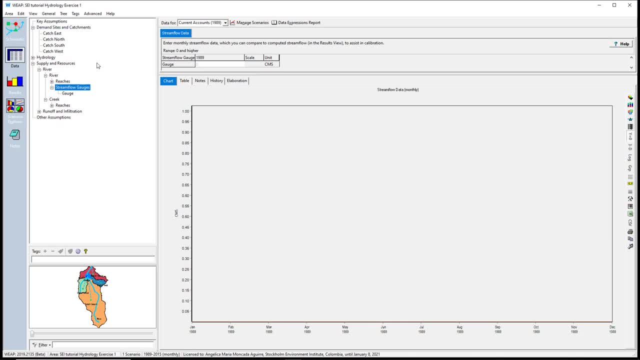 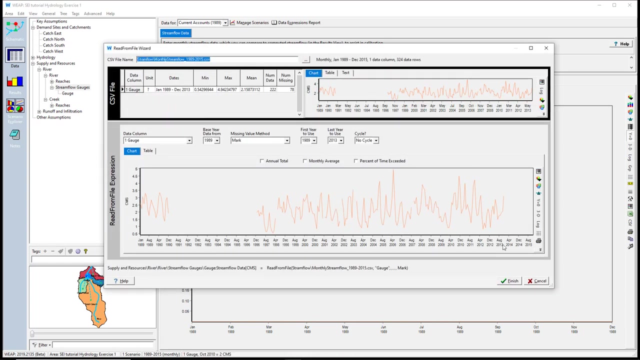 You can then go to the variable directly in the data view using the data tree Select read from file. wizard for entering the streamflow information. Access the streamflow folder and select the file monthly streamflow 1989- 2015.. The file has monthly information. Check the text tab. 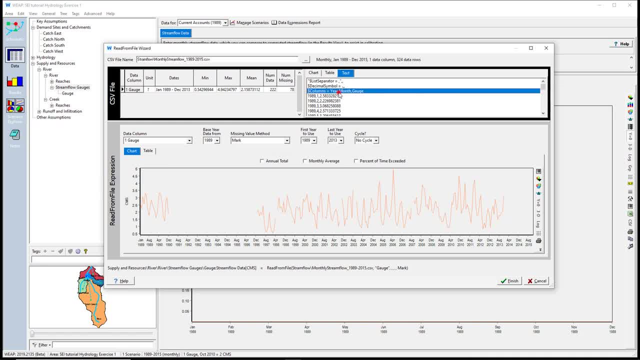 The file has three columns named year, month and gauge. We can see the information in the file. The graph shows missing data, but we will not use any method to fit the missing values. Finish Before continue entering the catchment information. 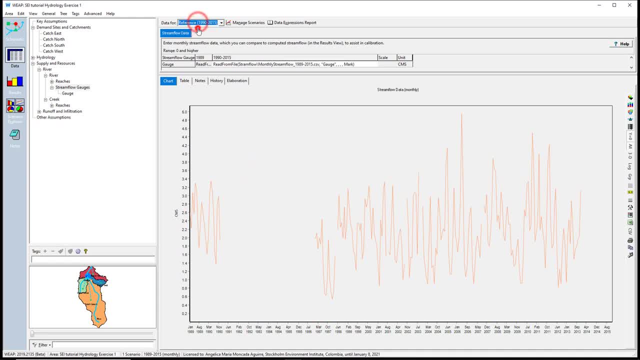 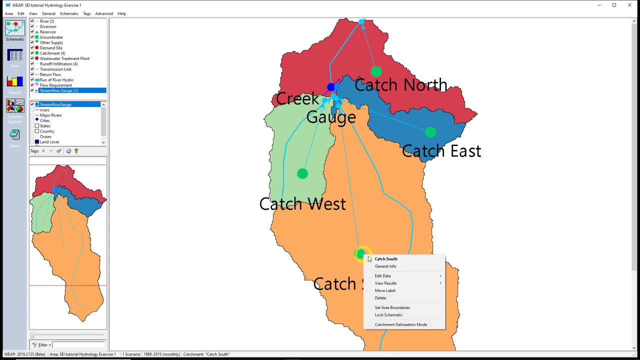 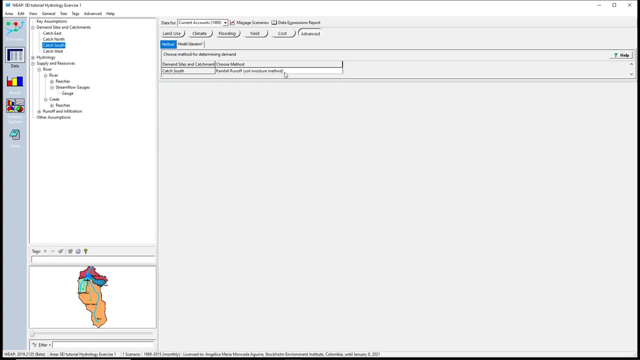 check the hydrological model. Select the hydrological method first. Go to the schematic view. Right click on any catchment, for example catch south. Select, edit data and then method. The method selected is the soil moisture method. Check the method of the other catchments. 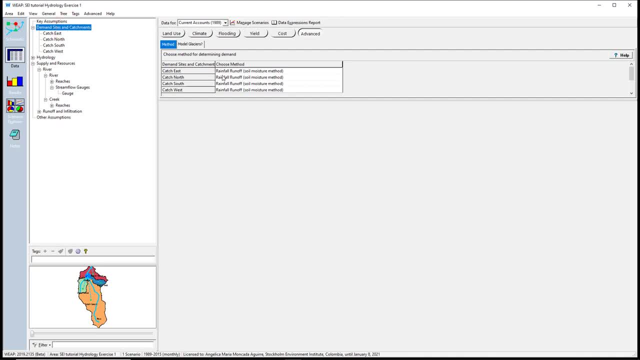 Click on demand sites and catchments. All catchments have the soil moisture method selected. We could change it here. We are going to continue entering the catchment information. The first step is to create the catchment disaggregation. Then we can enter areas. 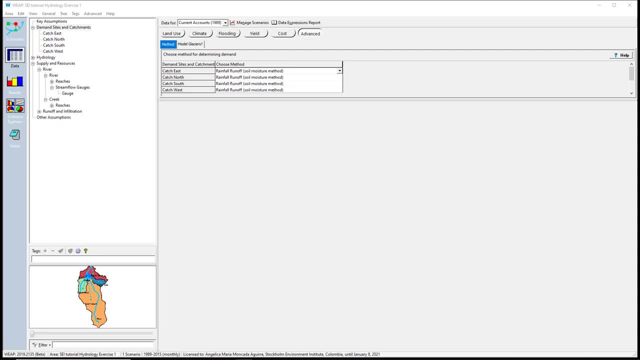 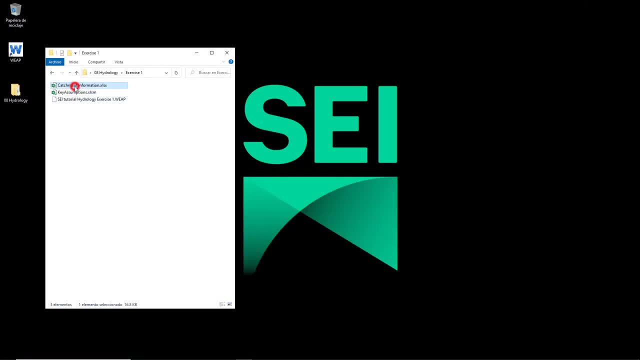 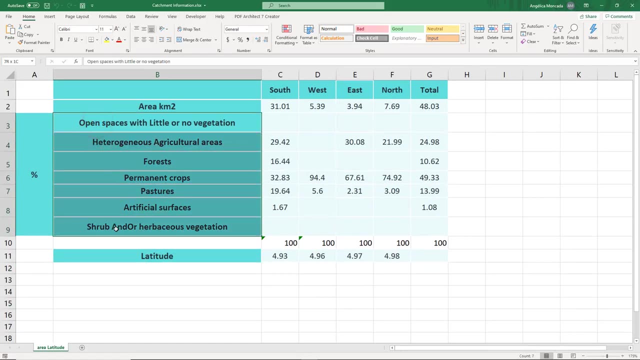 Finally, the climate and hydrological parameters are assigned to each catchment. Open the excel file- catchment information. We can see on the table that the catchment disaggregation is by land cover classes. The land cover classes are here in this column. 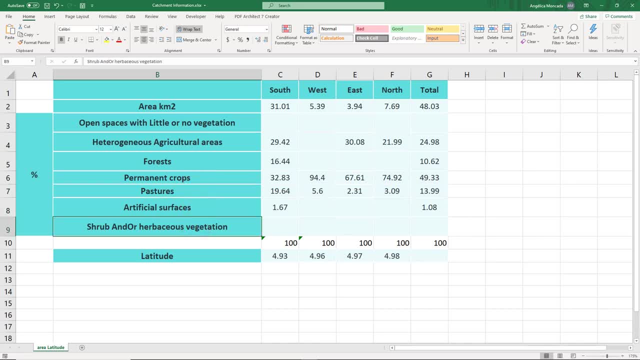 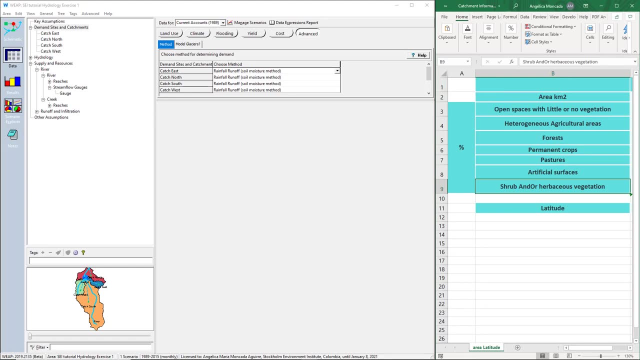 We must create these classes in WIP. under each catchment, Copy the name of the first land cover class from the excel file: Open spaces with little or no vegetation. Go to the first catchment, Right click on it and select add. We must enter a name. 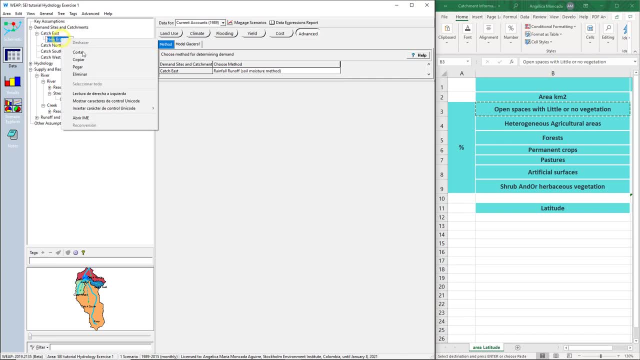 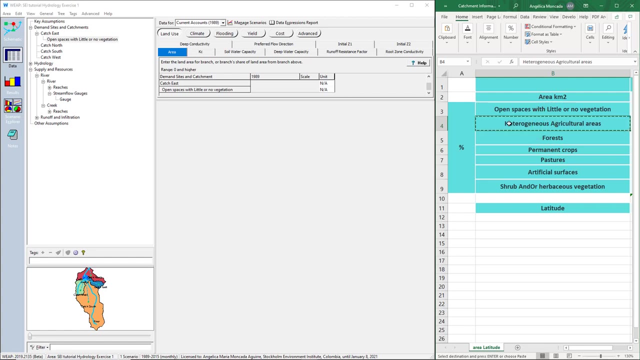 To paste the name in WIP, right click and select paste. The control V function does not work in WIP. Continue adding each class. Copy the name of the second class, heterogeneous agricultural areas, Then right click on the catchment and select add. 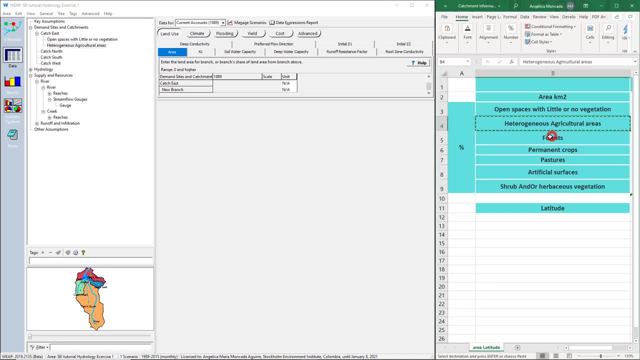 Right click and select paste Copy forests- Add. paste Copy permanent crops. Add paste Pastures. Artificial surfaces, Shrub and or herbaceous vegetation. Once we add the disaggregation, in this case by land cover classes, we can enter the areas. 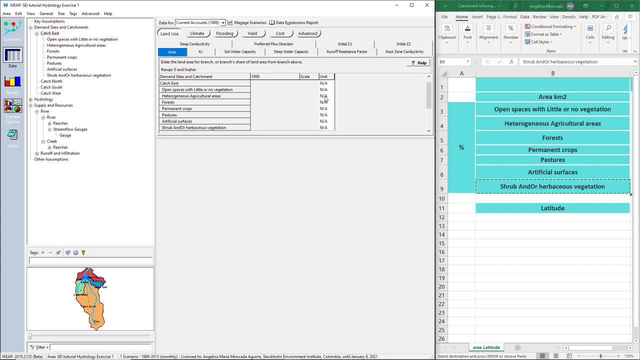 Go to the area variable. We need to assign the unit first for entering the data. We will enter the total area in the first box and the percentage distribution by land cover classes in the rest of the boxes. Select square kilometers for the area and percentage for the land cover classes. 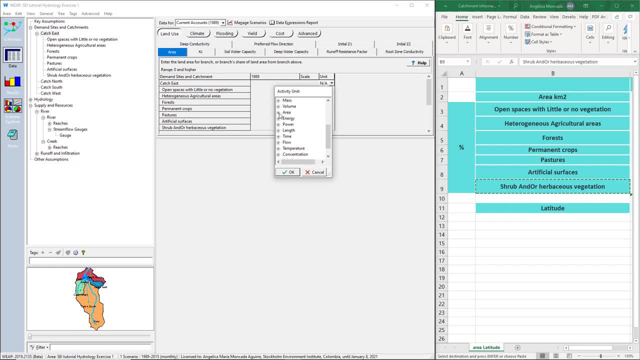 In the first box under unit, select area- square kilometers from the drop down menu. In the rest of the boxes, select share. This disaggregation is made the first time manually. We do not have to repeat this process. We can copy and paste these branches to other catchments. 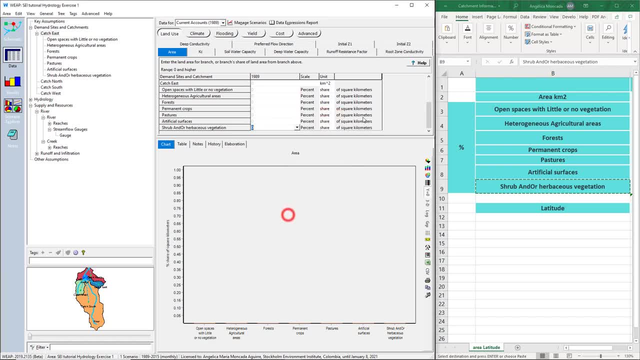 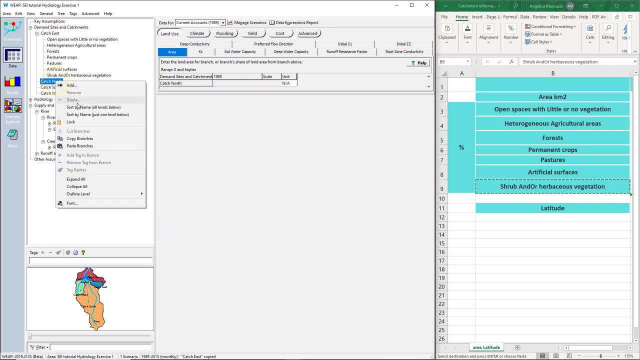 We need to have first this empty structure created, Then select the catchment with the empty structure, Right click on it and select copy branches. Right click on the catchment to which you want to paste the branches and select paste branches. We can repeat this process as many times as we need. 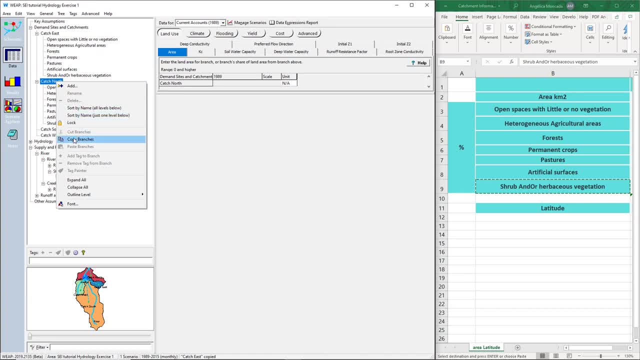 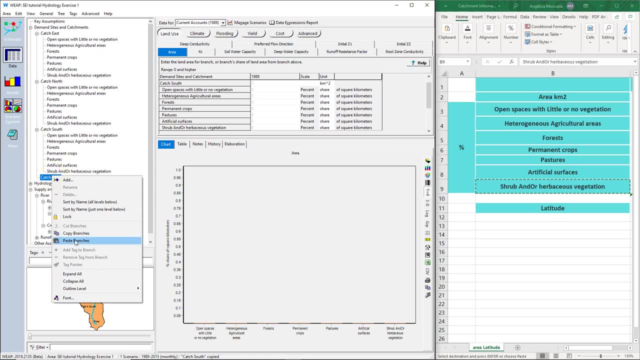 Do the same for the other two catchments: Copy branches, Paste branches, Copy and paste. The first time is manual. Then we can copy and paste the branches. We can finally enter the information. We will do it by exchanging the information with Excel. 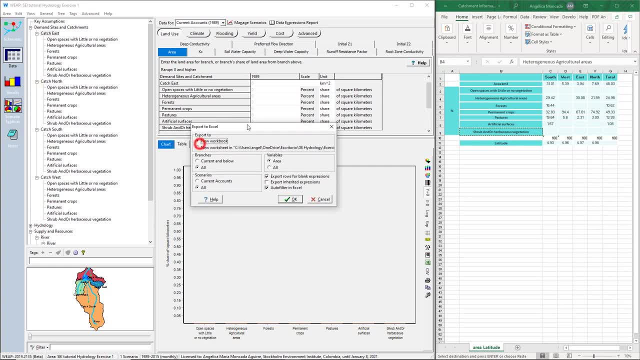 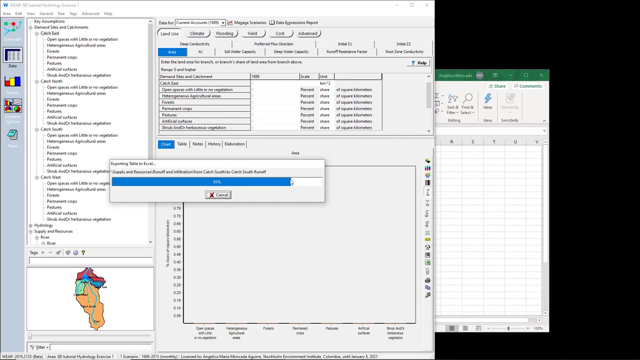 Go to Edit Export Expressions to Excel. We want the area variable for now. Select Export to New Workbook Branches: All Scenarios, Current Accounts, Variables Area. OK, We can assign the expression in this file to the element variable. We can assign the expression in this file to the element variable. 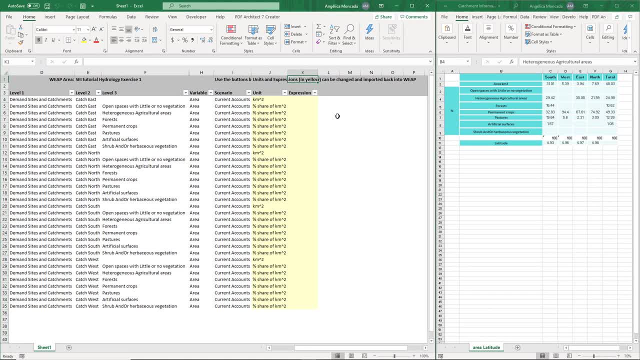 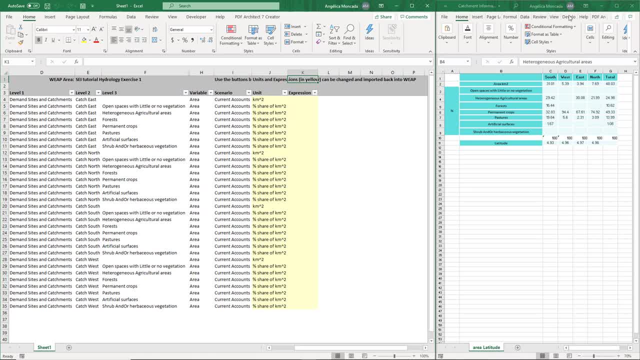 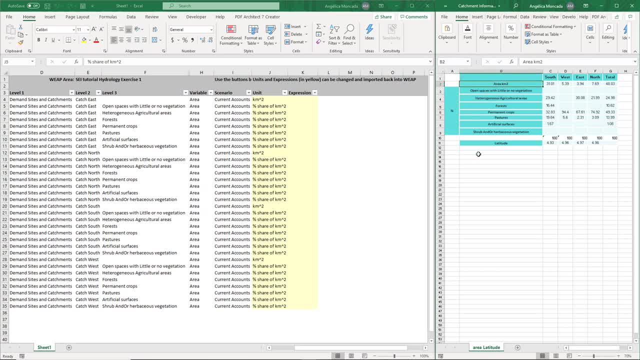 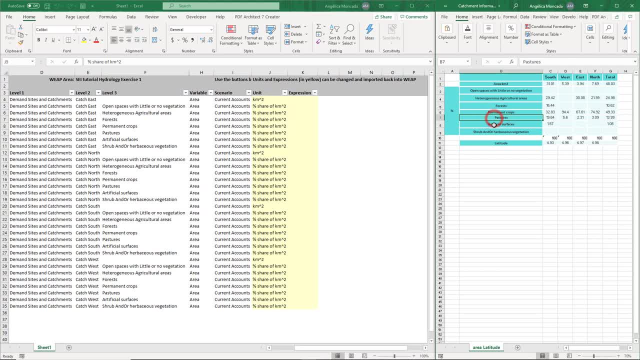 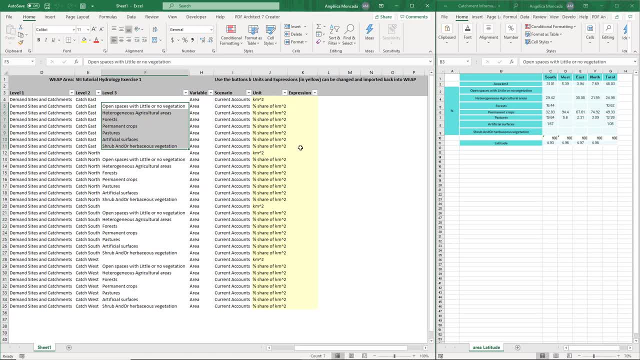 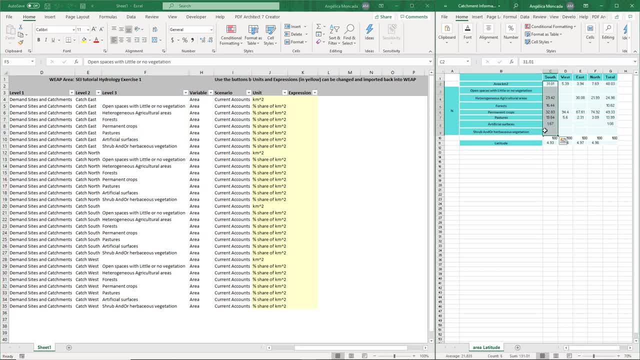 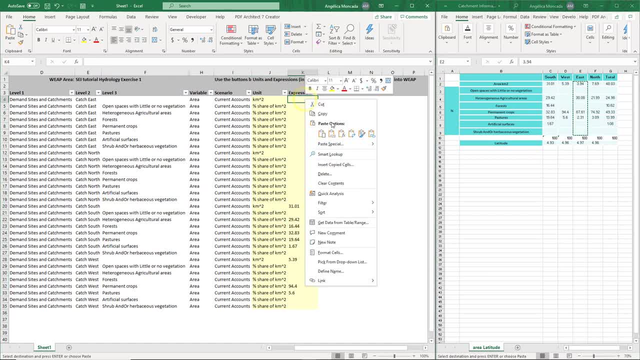 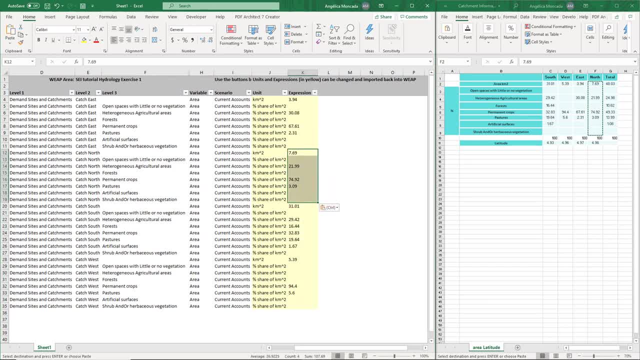 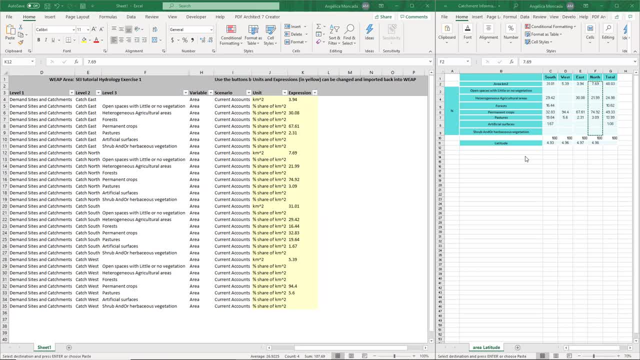 The units in the file are OK. The units in the file are OK. The units in the file are OK. The process for assumption is the same as before. If VIV is様's function and if its function is Masa's, Then the summation must be exactly. 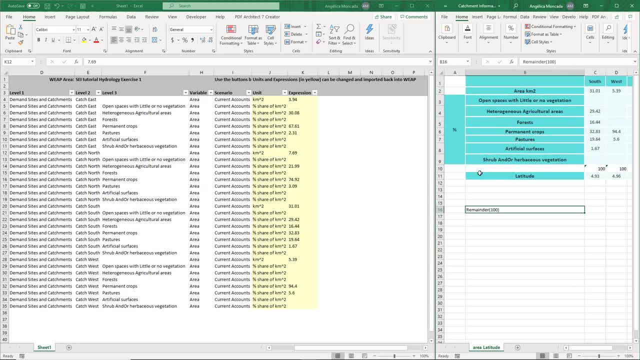 100%. To ensure that the sum is 100%, we can use the remainder 100 function in one land cover class. The remainder 100 error is to calculate a category automatically. What VIV is going to do is assign the missing percentage to reach 100% to the land cover class in which the 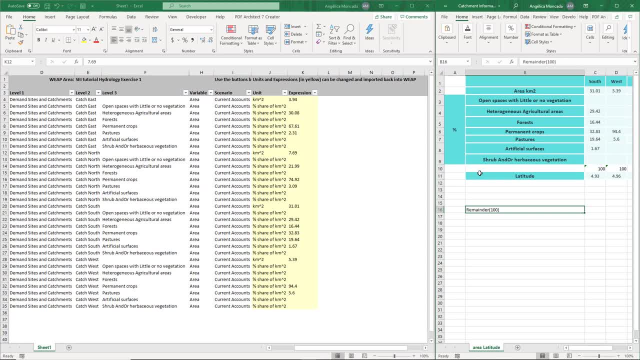 function was assigned. We could add the function in any land cover class. However, if you are going to include scenarios of land cover changes, it will be better to use the function in the land cover class that will be changed. For example, if it is a reforestation scenario, we could use the function in the forest or 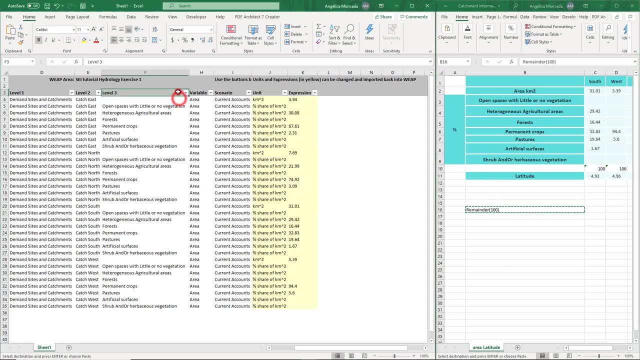 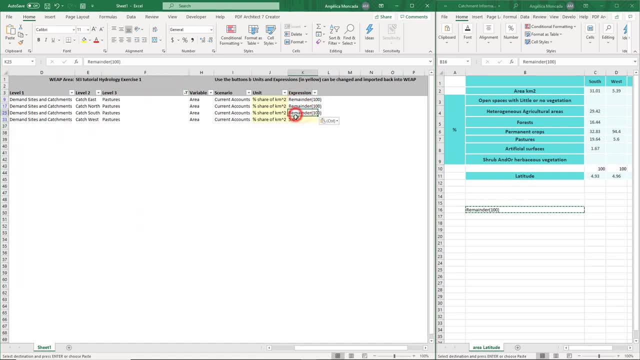 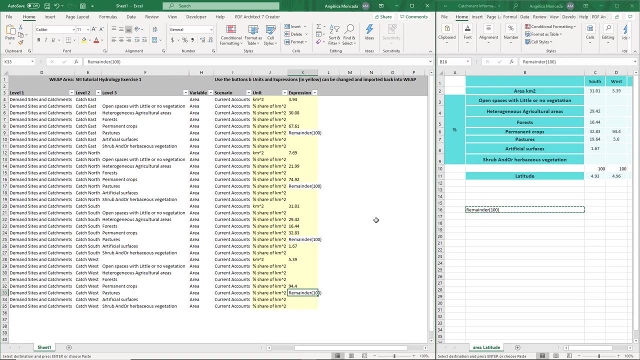 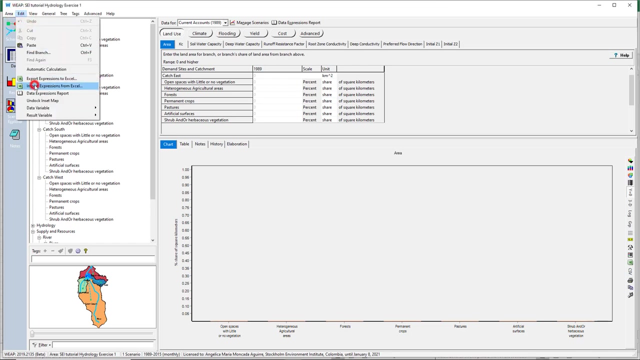 pasture classes. Use the remainder100 function in the pasture class. Change the value to remainder100.. You should now have the information like this: Go to Weep to import these expressions. Go to Edit: Import Expressions from Excel. Always check from which file Weep will import the information. 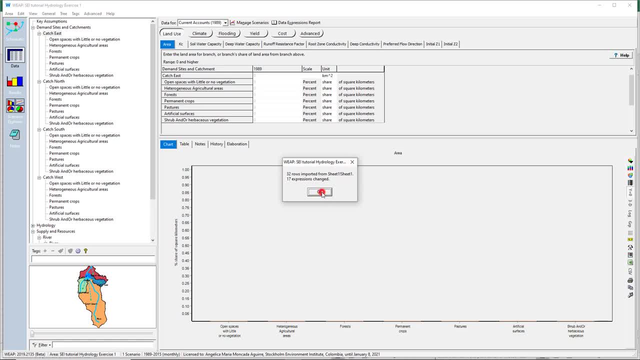 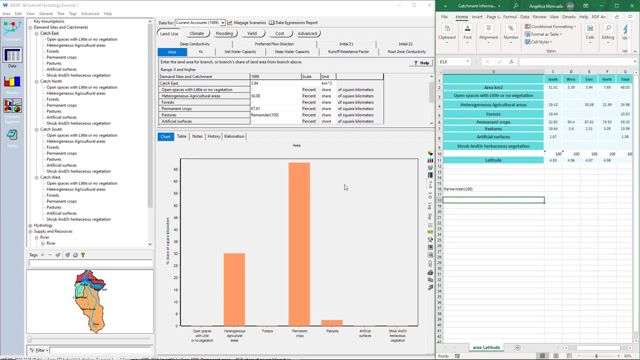 Once Weep finishes, we will be able to import the information. Go to Edit Import Expressions from Excel. Once Weep finishes, it shows a summary. Verify that the information we entered in Excel was imported. In the Cache North catchment we have 7.69 km2, 21.99% of heterogeneous agricultural. 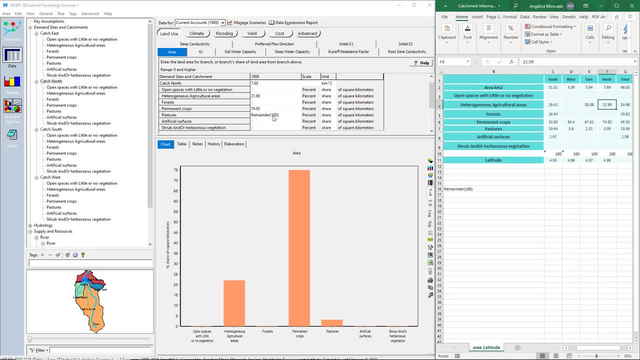 areas 74.92% of permanent crops. The remaining percentage will be pastures. The remainder 100 function should calculate 3.0.9%. We can go to the table to check. There is 3.1% of pastures. 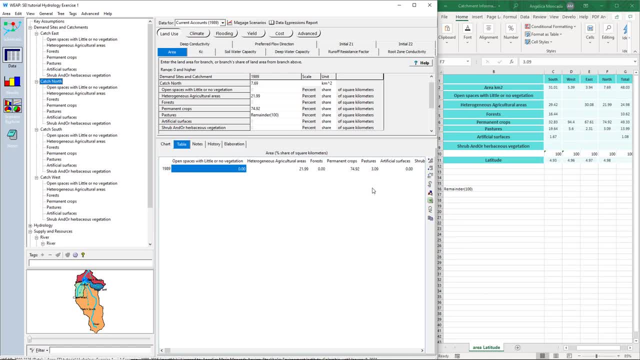 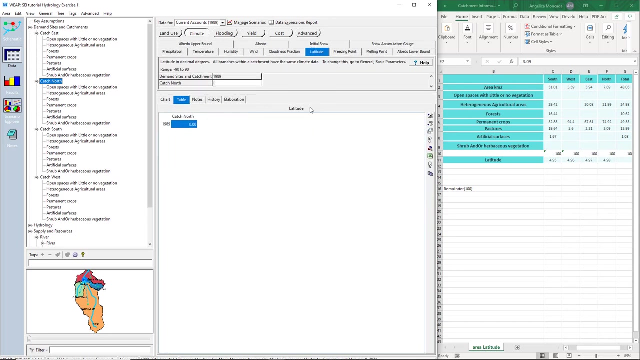 The remainder 100 function is useful for entering percentage distributions to ensure that all the entered values safe. Let's have a look at the table. sum: exactly 100 percent. we are going to continue adding the latitude information. go to the latitude variable under the client tab for the demon sites and catchments. go to edit export expressions to. 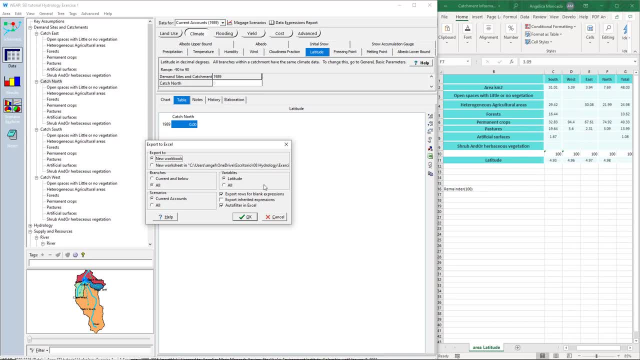 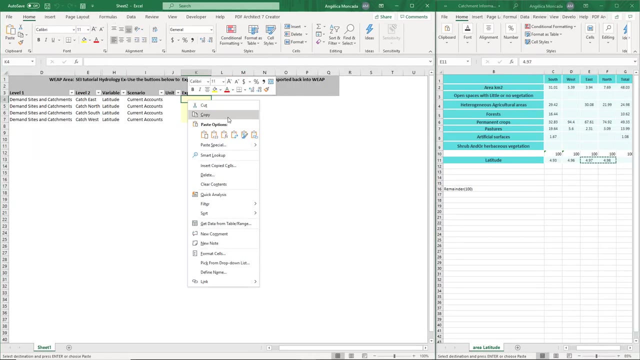 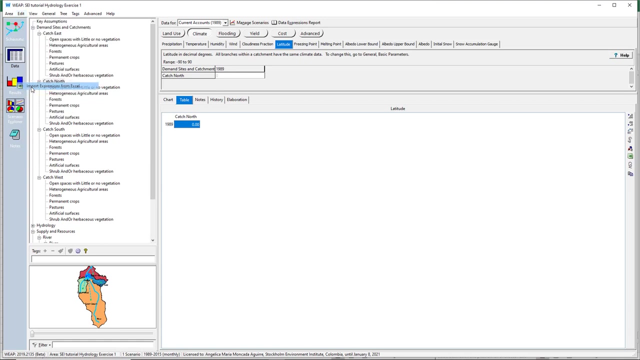 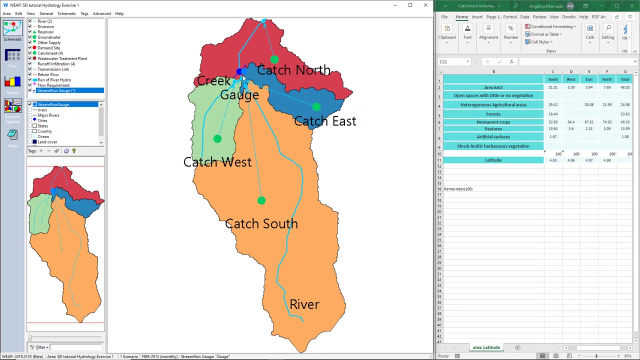 excel. we want the latitude variable: select, export to new workbook branches. all scenarios: current accounts, variables, light. the information is in the file. catchment information. verify the order of the information. copy and paste it. go to edit import expressions from excel. verify that the data were imported. we have already entered the elements: reverse catchments, runoff, infiltration links. 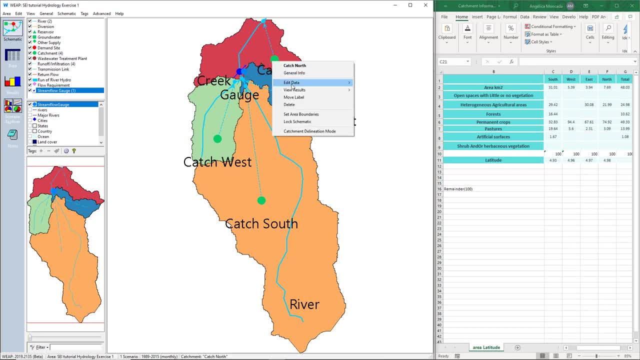 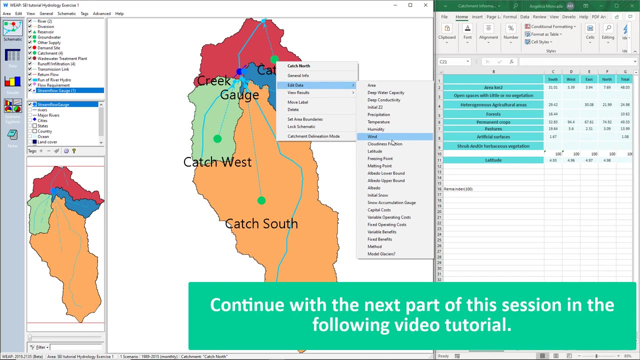 and a streamflow gate. we also enter the area and latitude for each catchment and the streamflow to the gauge. we will continue in the next session entering the climate data, creating key assumptions using a script, linking them to the hydrological parameters and exploring the results. so. 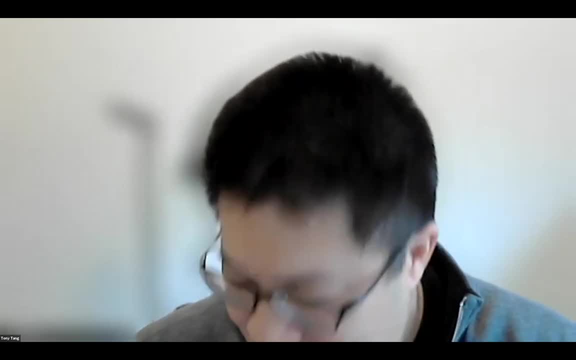 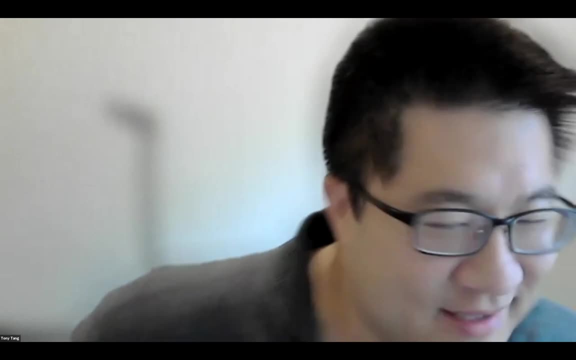 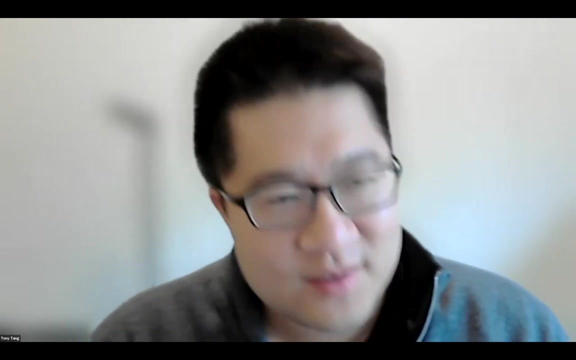 So, for those of you joining us, we're going to get started maybe in about a minute or two. If you're wondering why the Olympics music is playing, it's because we thought it'd be funny to have some background music, So I'm going to leave that playing for another minute or so. 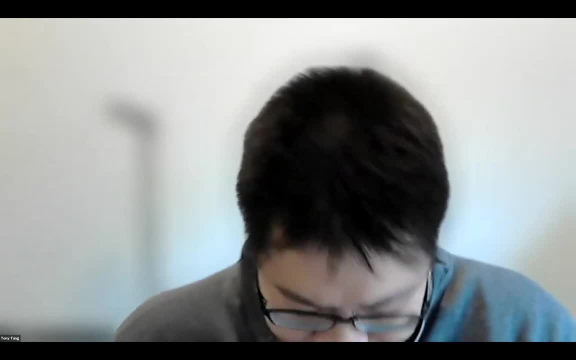 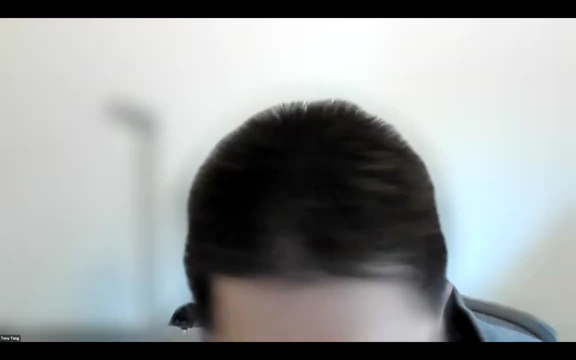 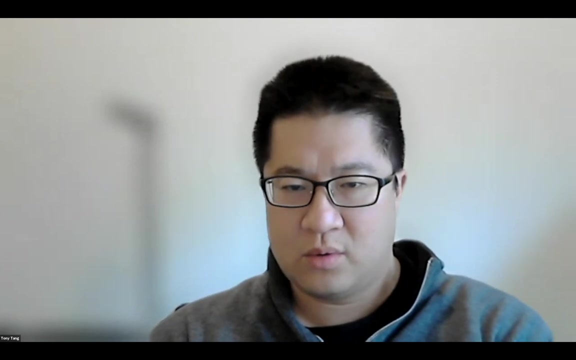 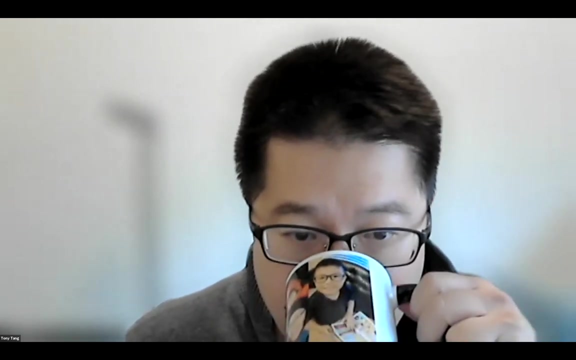 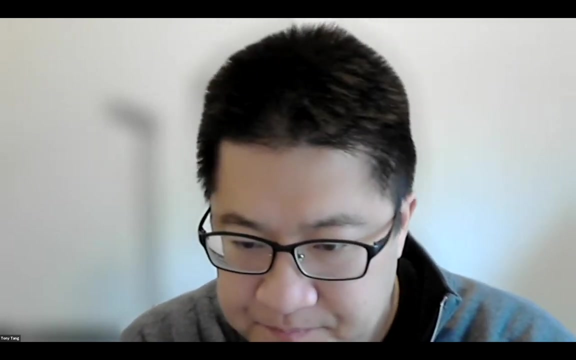 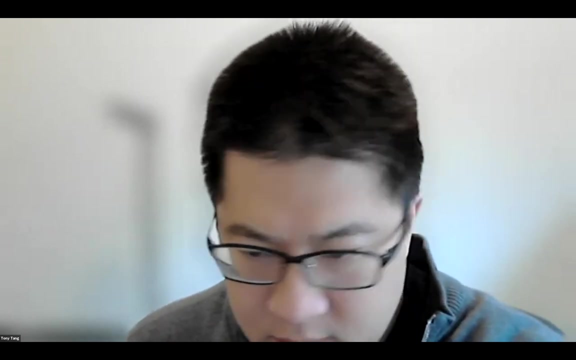 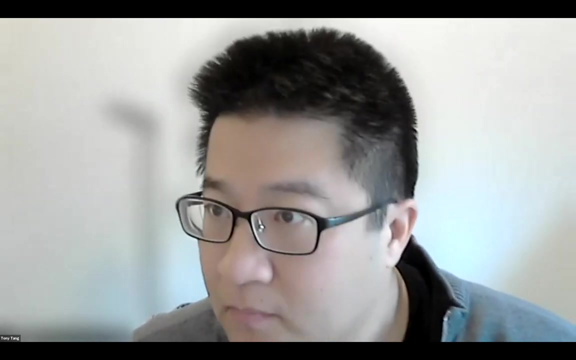 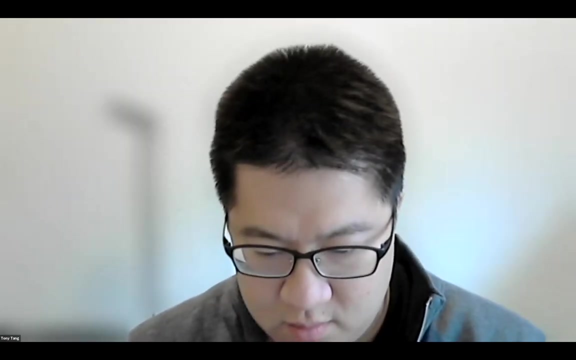 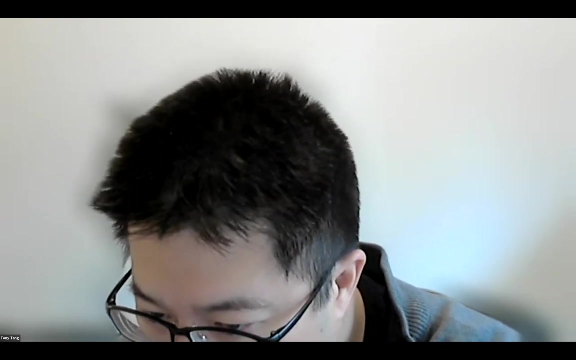 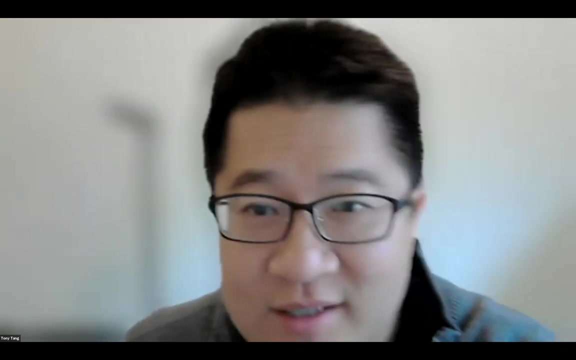 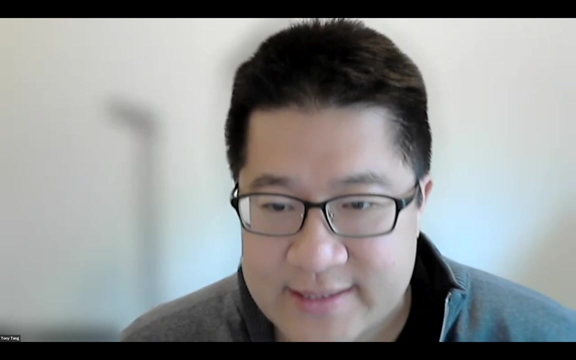 Just wait for stragglers to join us. Okay, so we're going to get started in about a minute or two. All right, Welcome to folks that are joining us today. Thank you so much for meeting us in this session. This is a session that is going to run for an hour. It's called Human-Computer Interaction. 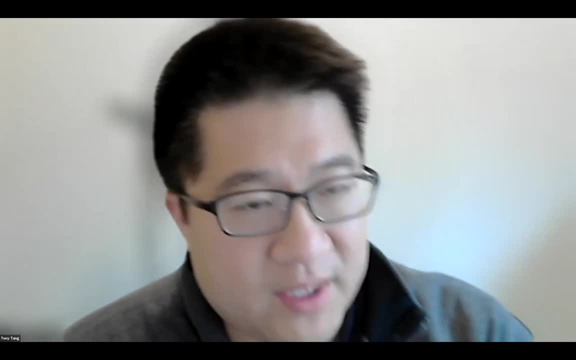 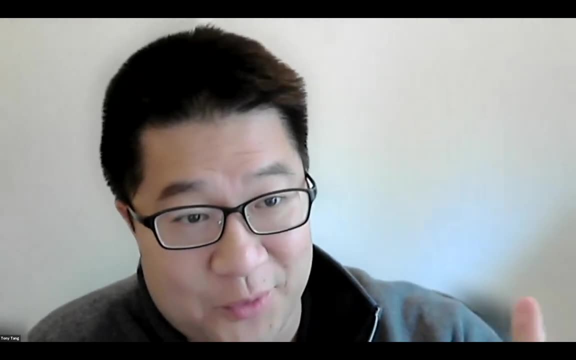 and User Interface Design. It's hosted by me. My name is Tony Tang, I'm an associate professor at the University of Toronto And my colleague, if you want to introduce yourself. Hi everyone, I'm Anastasia Puzmini. I'm also a professor.